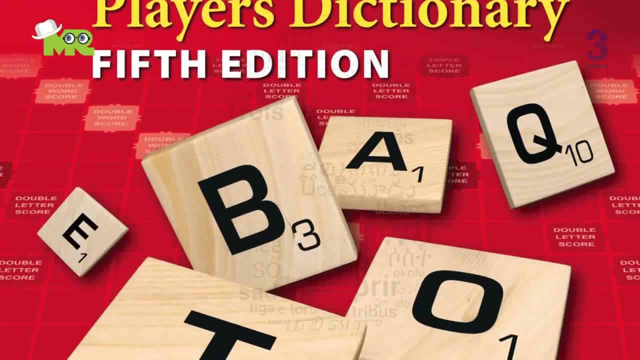 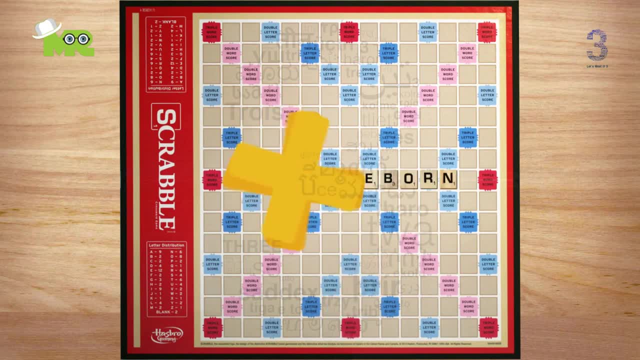 There are also official Scrabble dictionaries that can be purchased for more word options. There are some words that are not allowed to be played, and these include suffixes, prefixes and abbreviations. Any word that requires the use of a hyphen or apostrophe. 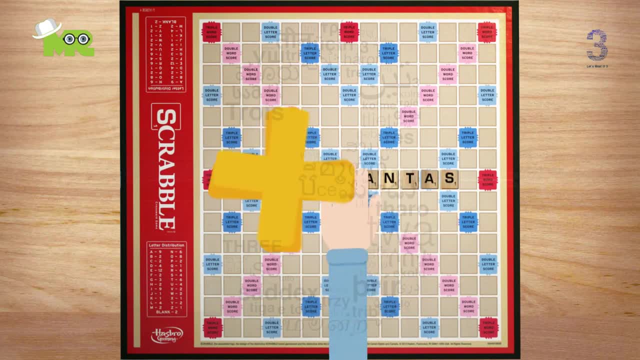 cannot be played in the game. Any word that requires the use of a capital letter is not allowed. When playing an English version of the game, foreign words are not allowed to be placed on the board. However, if the foreign word does appear in the standard English dictionary, it is allowed. 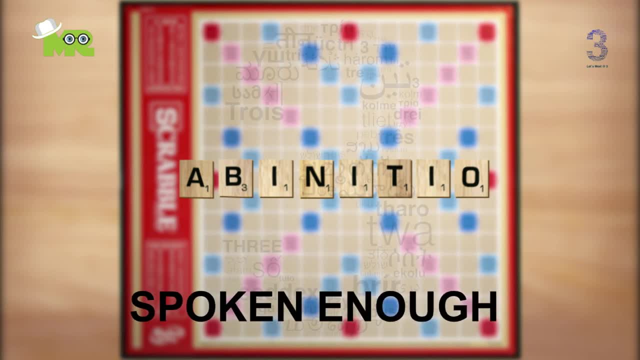 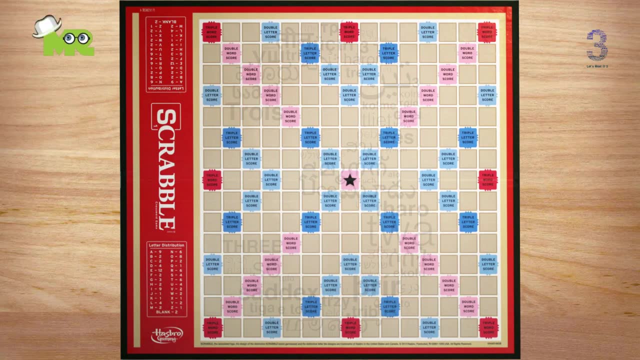 The reason for this is due to the fact that the word is spoken enough and is considered part of the English language. Extra point values: When looking at the board, players will see that some squares offer multipliers. Should a tile be placed on these squares, the value of the tile will be multiplied by two times or three times. 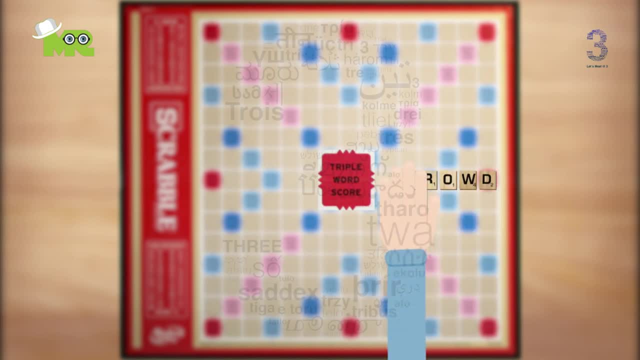 Some squares will also multiply the total value of the word and not just the single point value of one tile. Double letter scores: The light blue cells in the board are isolated and when they are used they will double the value of the tile placed on the square. 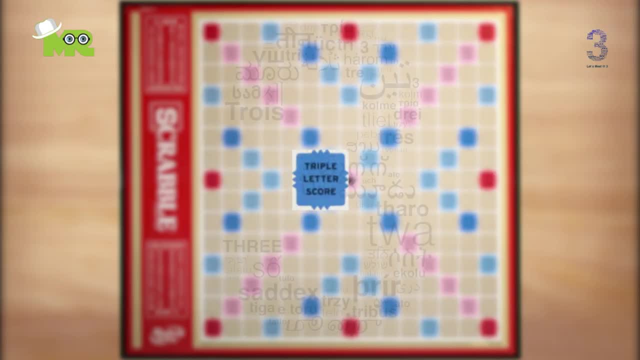 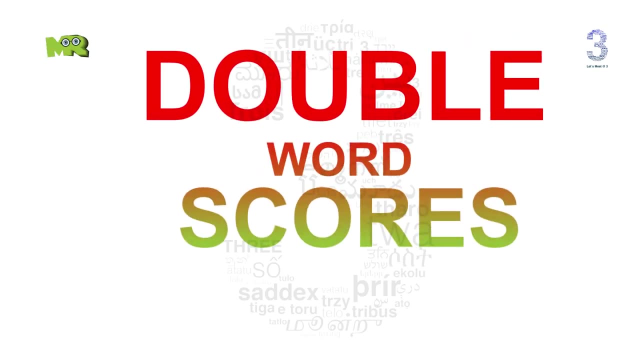 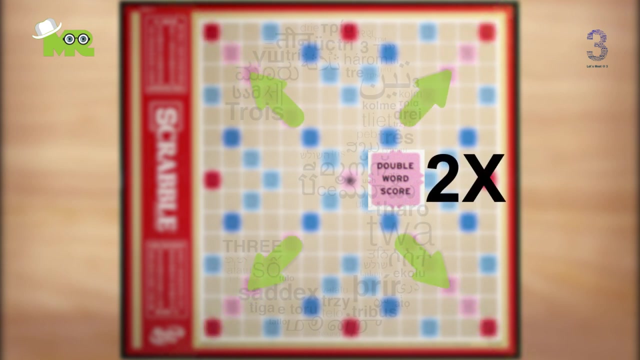 Triple letter score. The dark blue cell in the board will be worth triple the amount, so any tile placed here will earn more points. Double word score: When a cell is in light red in color it is a double word cell and these run diagonally on the board towards the four corners. 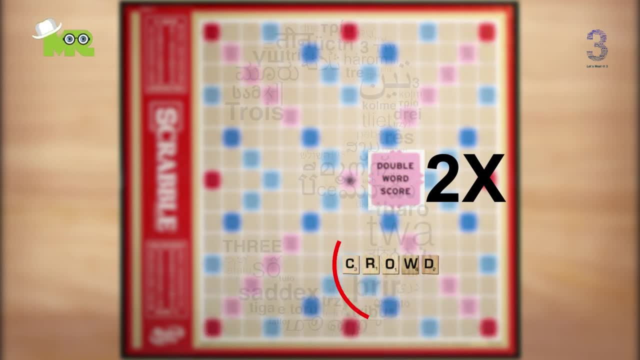 When a word is placed on these squares, the entire value of the word will be doubled. Triple word score. The dark red square is where the high points can be earned, as this will triple the value of the word. These are found on all four sides of the board and are equidistant from the corners. 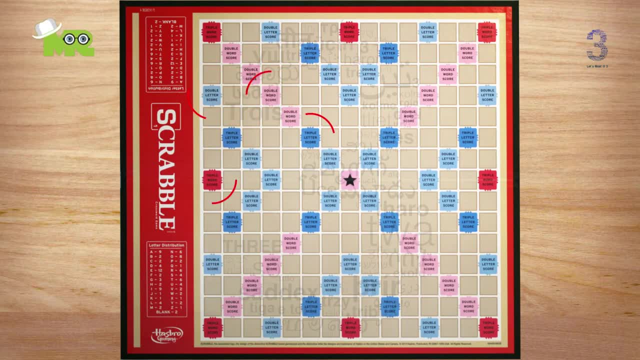 One single use When using the extra point squares on the board. they can only be used one time. If a player places a word here, it cannot be used as a multiplier by placing another word on the same square. Let's start the game. 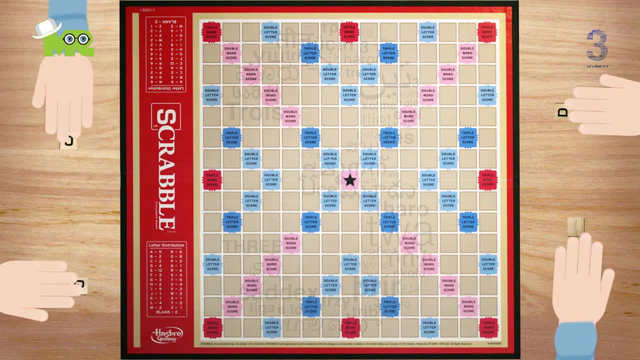 Choose one player to be the scorekeeper. Everyone draws one tile. The player with the letter closest to A goes first. The blank tile automatically goes first. Now each player draws seven letters from the Scrabble bag and places them on your letter rack. 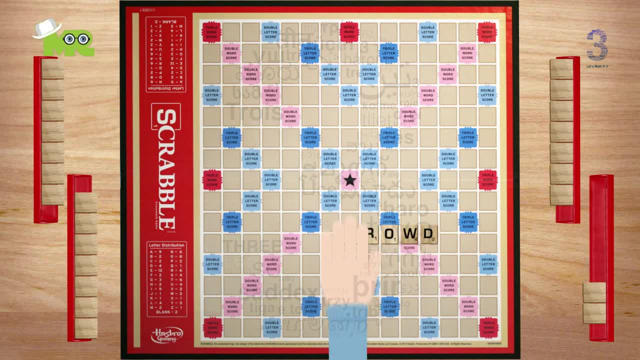 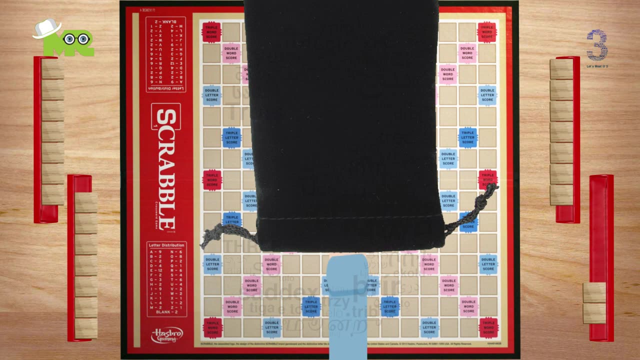 There are three options during any turn. The player can place a word, they can exchange tiles for new tiles or they can choose to pass. In most cases, players will place a word, as the other two options will result in no score. When a player chooses to exchange tiles, they can choose to exchange one or all of the tiles they currently hold. 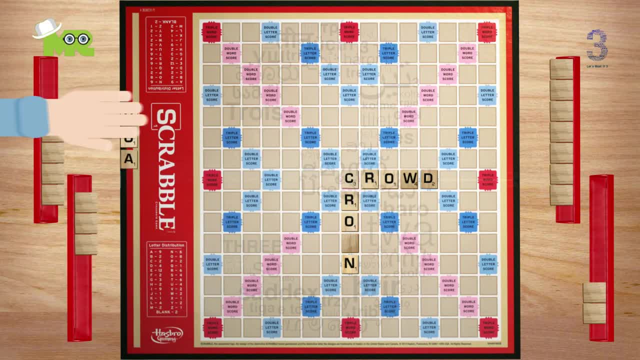 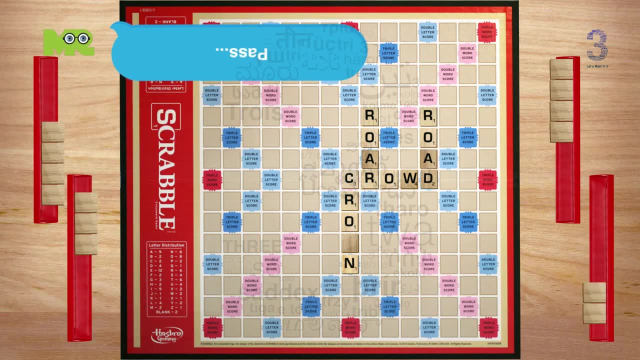 After tiles are exchanged, the turn is over and players will have to wait until their next turn to place a word on the board. Players can choose to pass at any time. They will forfeit that turn and hope to be able to play the next time. 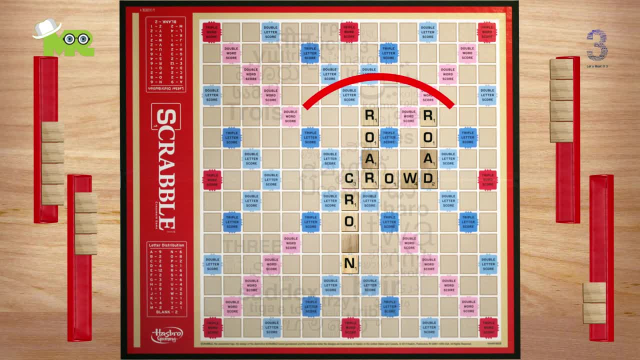 No tile may be moved or replaced after it has been played. But if you own the tile with the letter that the blank tile is being used for, you can take the blank tile by substituting your tile for the blank tile on the board. Any player may challenge a word before the next player starts their turn. 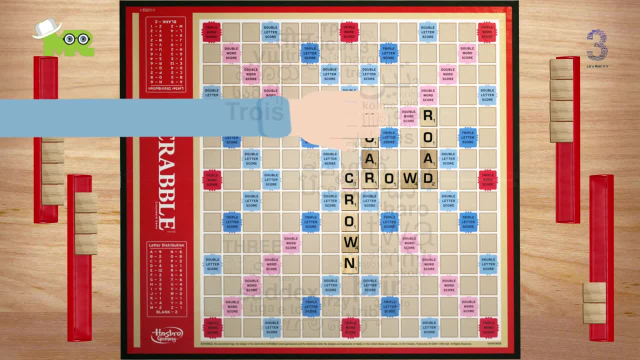 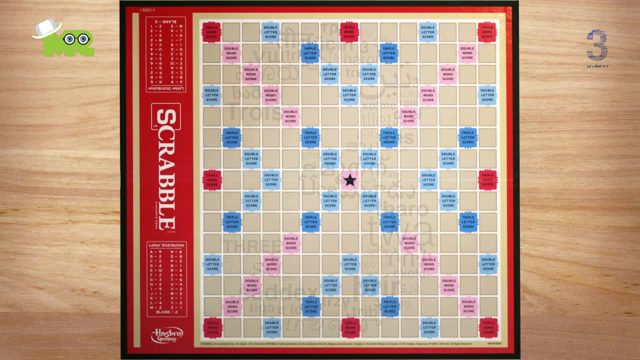 If your word is not in the dictionary, you must take back your tiles. This ends your turn. The First Word Score. When the game begins, the first player will place their word on the star spin in the center of the board. The star is a double square and will offer a double word score. 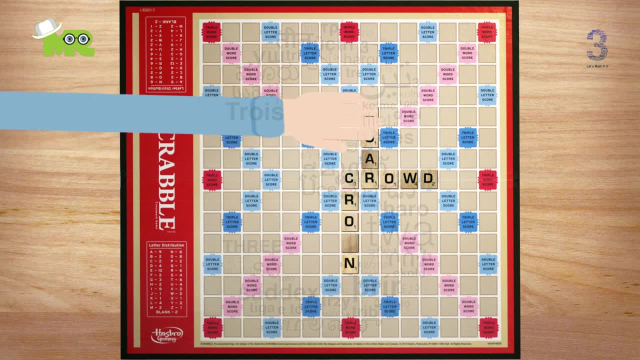 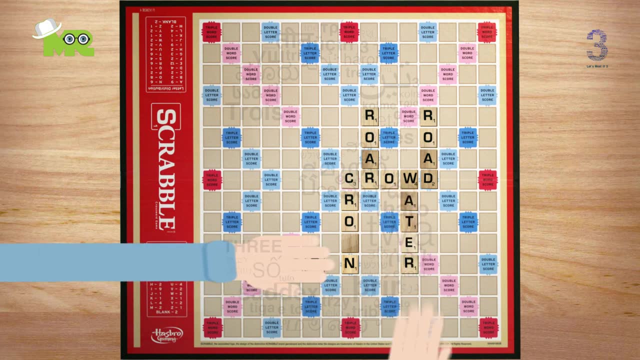 All players following will build their words off of this word, extending the game to the other squares on the board. All touching letter tiles must form complete words. Play continues in a clockwise direction around the Scrabble board When you can replace Scrabble tiles. 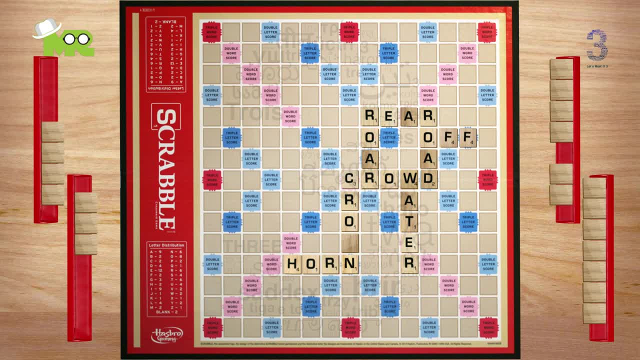 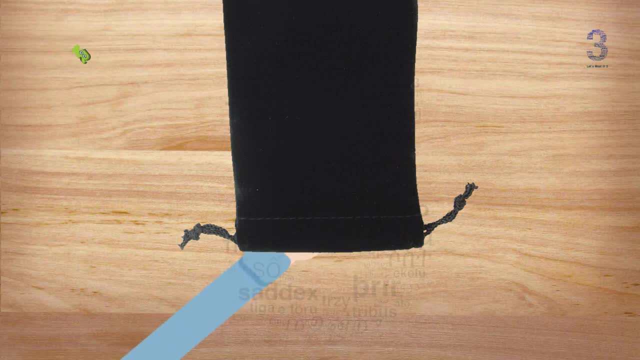 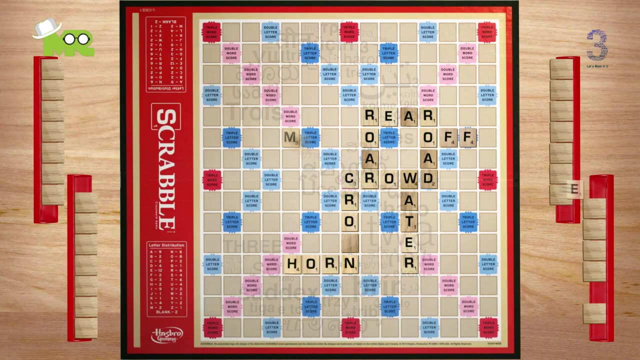 Once tiles are placed on the board, players will draw new tiles to replace those. Players will always have seven tiles during the game. Drawing tiles is always done without looking into the bag, so that the letters are always unknown. Extra 50 points bonus: The player who uses all seven tiles to create a word on the board will receive a 50-point bonus in addition to the value of the word. 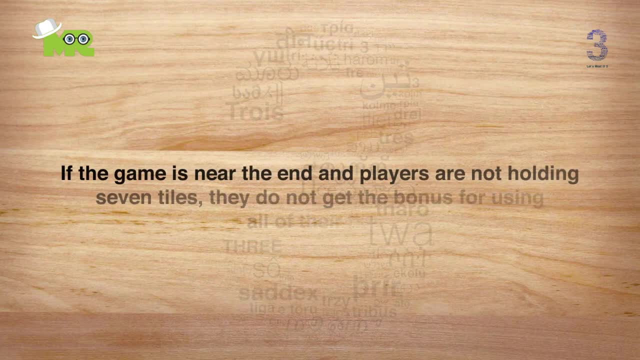 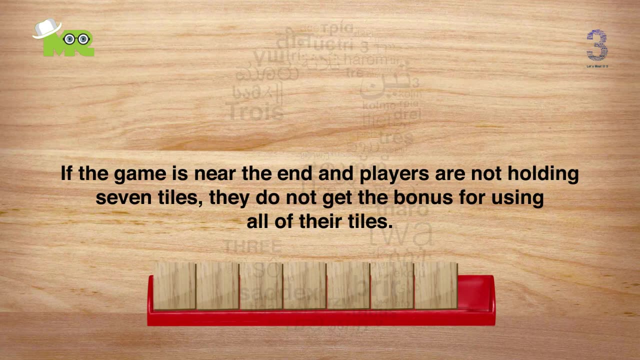 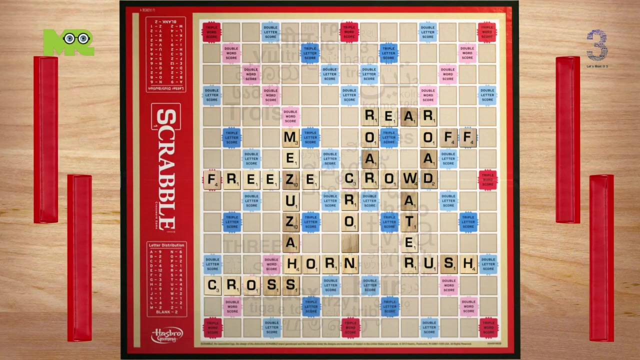 If the game is near the end and players are not holding seven tiles, they do not get the bonus for using all of their tiles. This is only collected for seven-letter words placed When the Scrabble game ends, Once all the tiles are gone from the bag and a single player has placed all of their tiles.